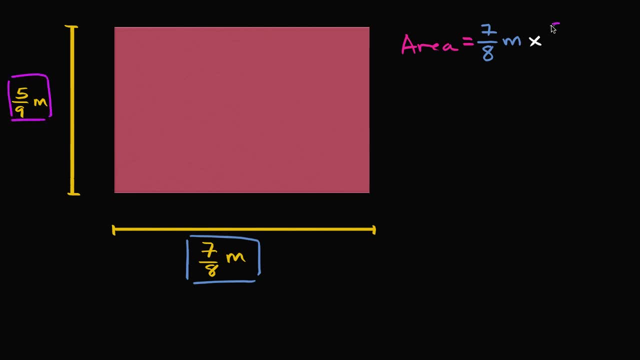 which is 5, 9ths of a meter. and what's that going to get us? Well, that's just going to be equal to the meters times. the meters give us square meters, So meters squared. We could write it like that: 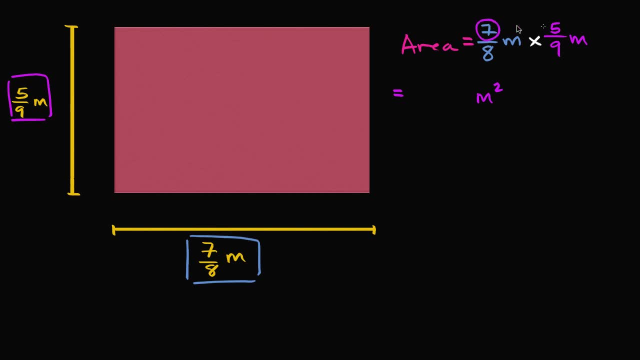 And then we're going to have 7 times 5 in the numerator to get us 35. And then in the denominator. In the denominator we are going to have 8 times 9 to give us 72. And we'd be done. 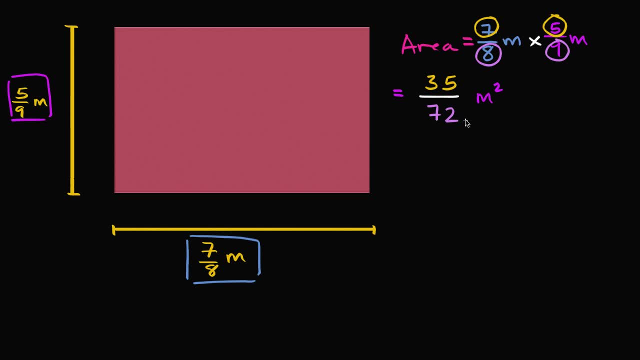 This is the area of this rectangle. here It's 35 72nds of a square meter. But what I want to do now is think a little bit deeper about why that actually makes sense, or just really another way of thinking about it. 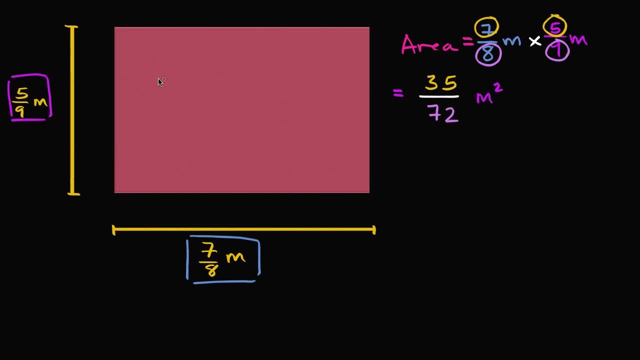 And to do that, what I'm going to do is I'm going to split this region into equal rectangles. So let's split it into equal rectangles And we see that we have 7.. If we go in the horizontal direction, we have 1,, 2,, 3,, 4,, 5,, 6, 7.. 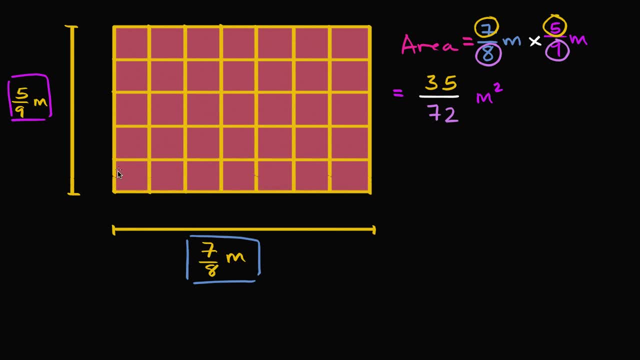 Or you could say: in each row we have 7 of these rectangles. In each column you have 1,, 2, 3, 4, 5 of these rectangles. So you can see we have 5 times 1,, 2,, 3,, 4,, 5, 6, 7.. 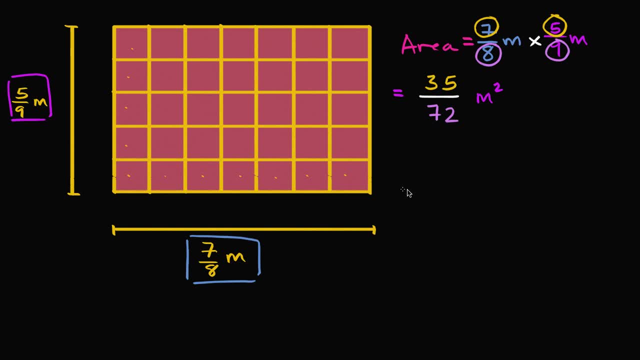 So we have 5 times 7 of these rectangles. So we have 35 rectangles. I'll just write it as 35 rectangles. And what's the area of each of those rectangles? Well, if this is 7 eighths meters wide, 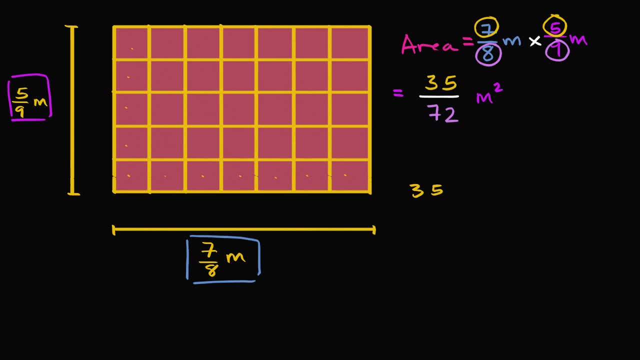 and this is divided into 7 equal sections in the horizontal direction. that means that each of these is exactly 1 eighth of a meter wide And, by that same logic, each of these, if this whole thing is 5 ninths and the height of each of these. 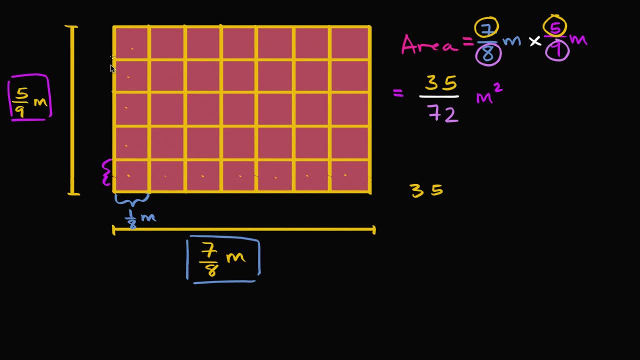 is 1 fifth, because we have 5 rectangles per column, then the height of each of these is going to be 1 ninth of a meter. So what's the area of just this character right over here? Well, it's going to be 1 ninth of a meter times 1 eighth.